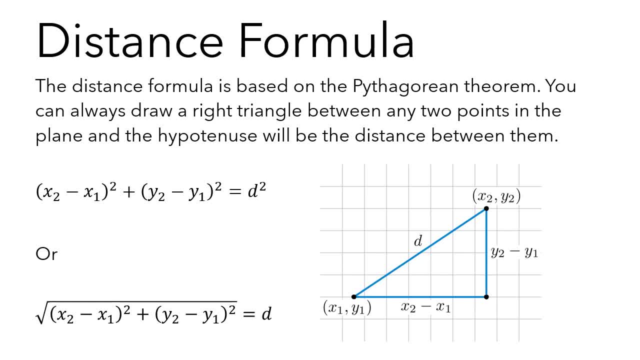 always draw a right triangle between any two points in the plane, The hypotenuse, which is just the longest side, c will be the distance between them. So notice, you've got a triangle over here. You've got this side, which is really just side a, then this side, which is really just 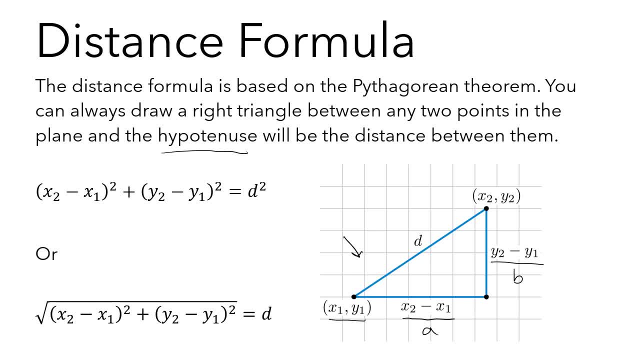 side b, Based on the coordinates x1, y1, and x2, y2, and then your hypotenuse is going to be side d, So it'd be a squared plus b squared. a squared plus b squared equals c squared, And you can. 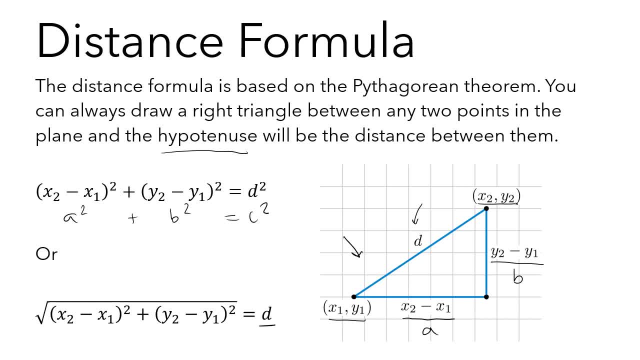 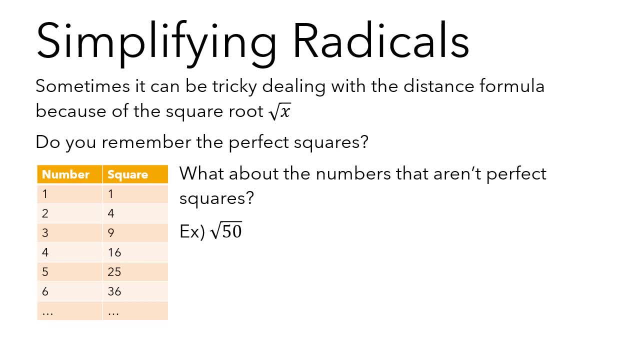 also write it with a square root where d is not squared, So this is what we call the distance formula. Sometimes, however, it can be tricky dealing with the distance formula because of the square root, So this is what we call the distance formula. 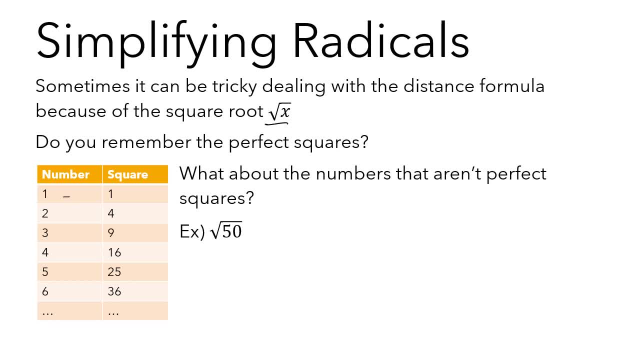 Do you remember perfect squares: 1 squared is 1,, 2 squared is 4, or 2 times 2,, 3 squared is 3 times 3 is 9,, 4 squared is 16,, 5 squared is 25, and 6 squared is 36, and vice versa. 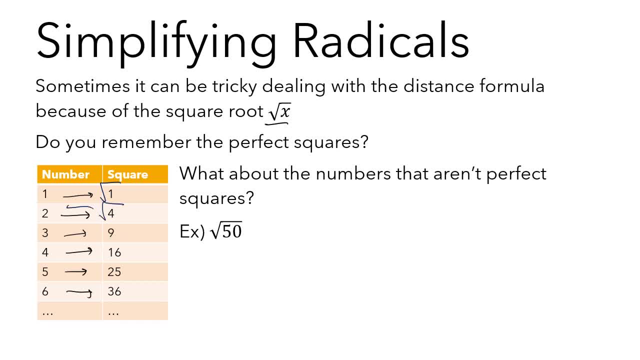 The square root of 1 is 1,, the square root of 4 is 2,, the square root of 9 is 3, so on and so on. It just goes backwards. Now those are perfect squares because they give you whole numbers. 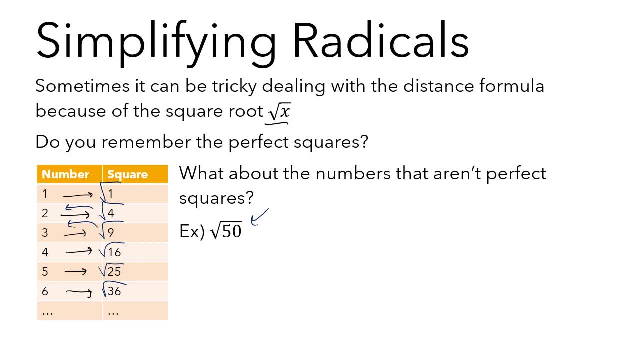 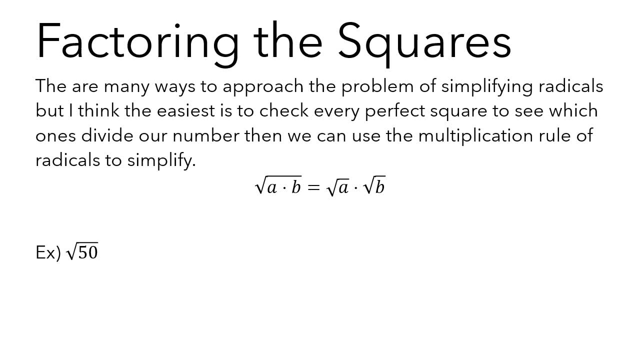 But what about numbers that aren't perfect squares, like the square root of 50?? We're going to have to deal with numbers like this. There are many ways to approach the problem of simplifying radicals, but I think the easiest is to check every perfect square to see which one divides our number. Then we can use the. 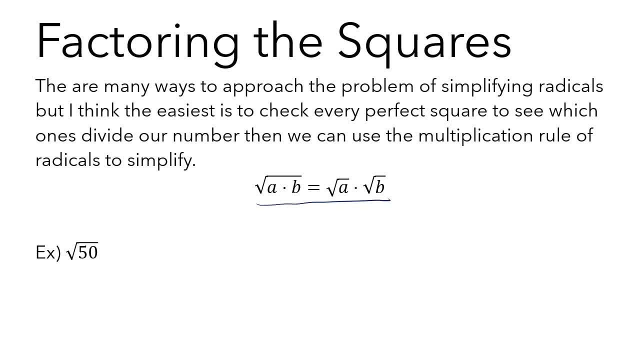 multiplication rule, which is this, namely that the square root of two numbers multiplied is the same thing as the square root of first number times the square root of the second one. to simplify our radicals, The square root of 50 is actually just the square root of 25 times 2, because 25 times. 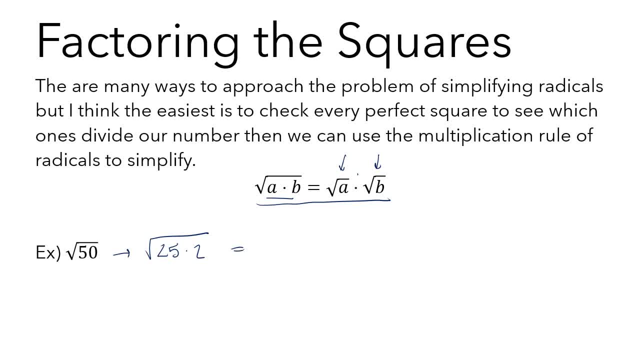 2 is 50, but 25 is the perfect square, So I'm going to split that using the multiplication rule to give me the square root of 25 times the square root of 2.. The square root of 25 is just 5, so this becomes 5 times the square root of 2, and this is considered simplified. 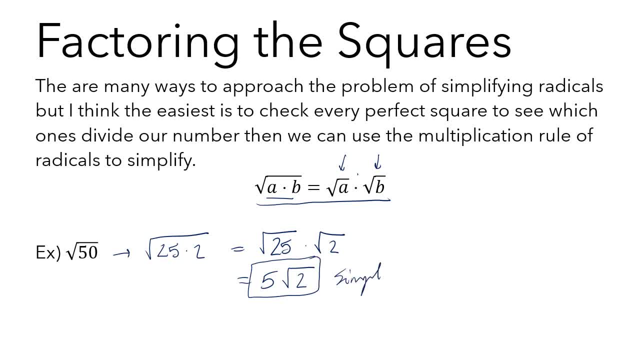 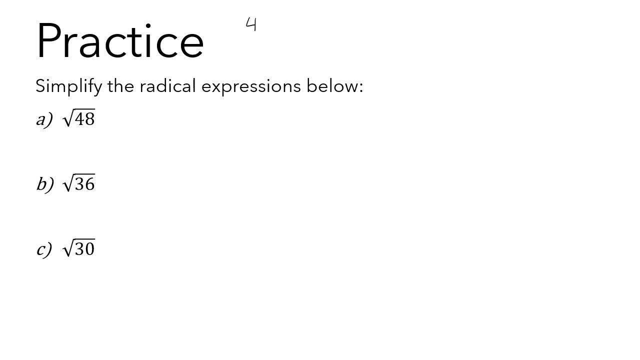 radical form. Let me write that out. This is considered simplified radical form. It's an important vocab word, So let's practice this. I'm going to start by writing out the perfect squares, So I'm going to start with 4,, 9,, 16,, and I'm going to keep going until I get to the biggest number. 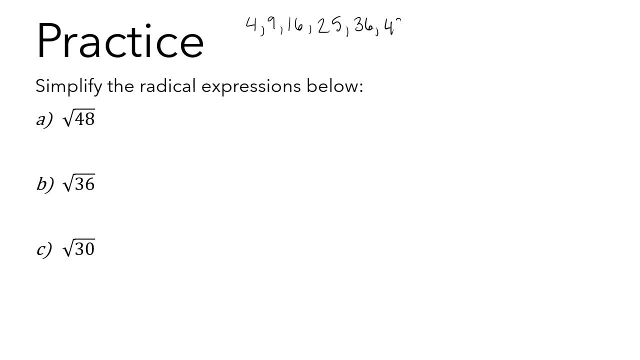 25,, 36,, then 49,, and that's bigger than any of the numbers I have. Okay, now I'm going to try and divide 48 by these perfect squares. Is 48 divisible by 36? No, Is it divisible? 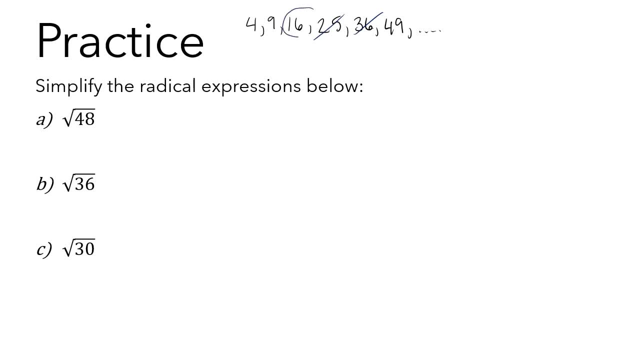 by 25? No. Is it divisible by 16? Yes, so the square root of 48 is actually equal to 16 times 3.. Now I can split that into the square root of 16 times the square root of 3, and that's. 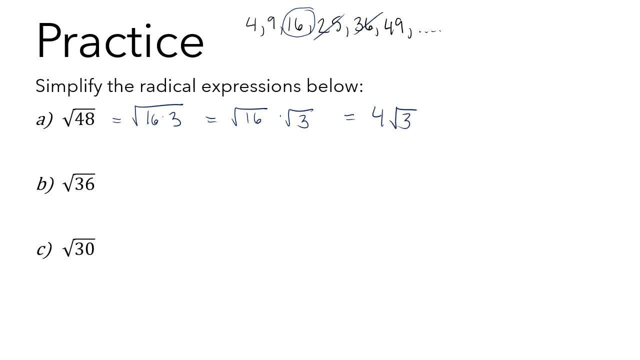 going to give me 4, square root 3, because the square root of 16 is just 4.. The next one is actually already a perfect square. My answer is going to be 6, so I'm done. Now the last one. I'm going to try again by dividing all the numbers. Of course, it's not divisible. 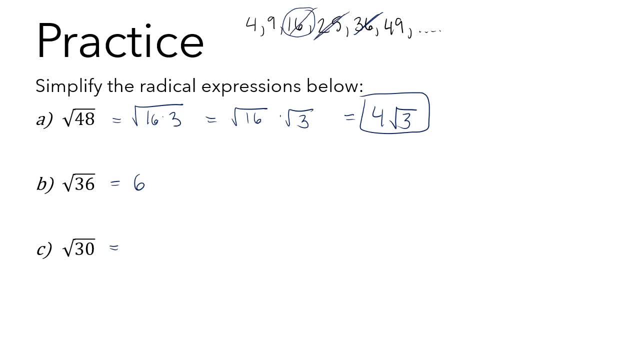 divisible by 36 or 25 or 16 or 9 or 4. so it turns out this is already in simplified radical form and I'm done. now let's use the distance formula and keep in mind that we will have to simplify into radical form. okay, so the distance formula, to remind you, is the 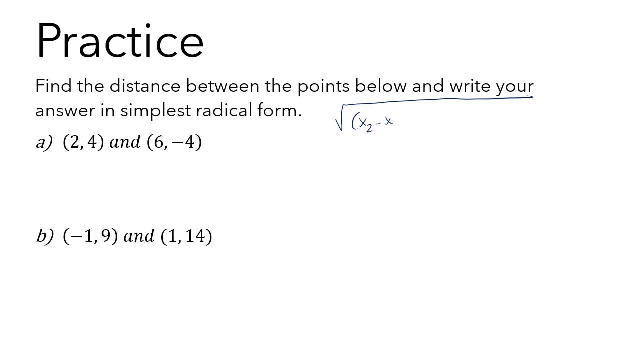 square roots of x2 minus x1 squared plus y2 minus y1 squared. so this is my x1- y1, x2, y2. so this is going to give me the square roots. x2 is 6, so 6 minus 2 squared, plus negative 4 minus 4 squared. 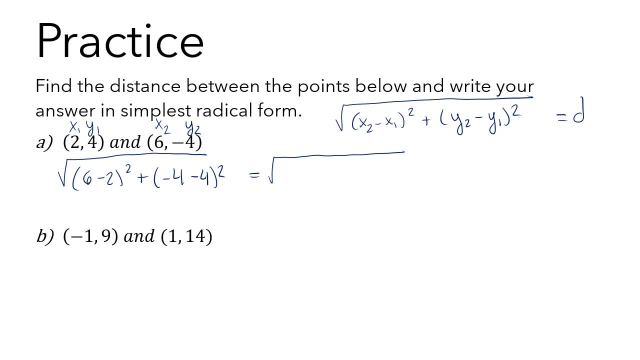 now that's going to equal: 6 minus 2 is 4, so I got 4 squared. and then negative 4 minus 4 is actually negative 8, so it's negative 8 squared. and then this is going to simplify to be: 4 squared is 16, negative 8 squared. keep in mind a.